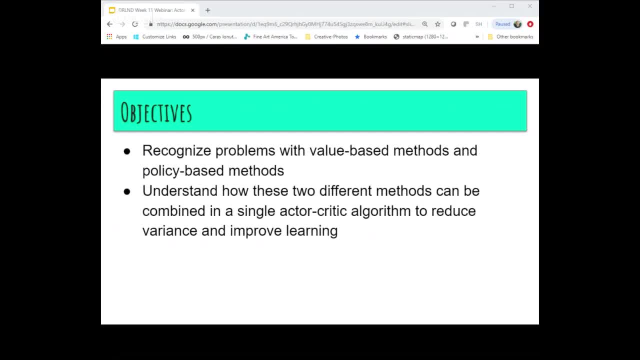 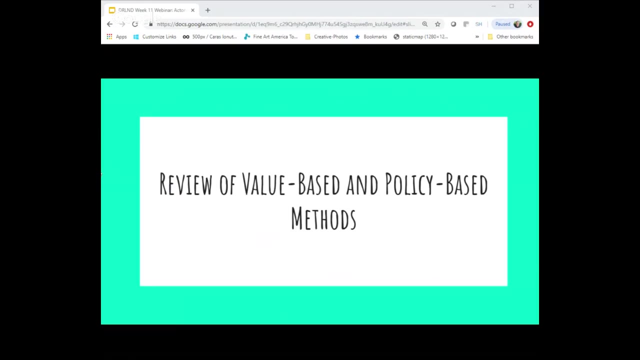 with the other two main methods we've talked about in the past- the value-based and the policy-based methods- and then to understand how these two different, independent methods can be combined into a single algorithm and thereby reduce variance and improve deep reinforcement learning. So here I start with a review of the basic value-based and policy-based methods. So we've 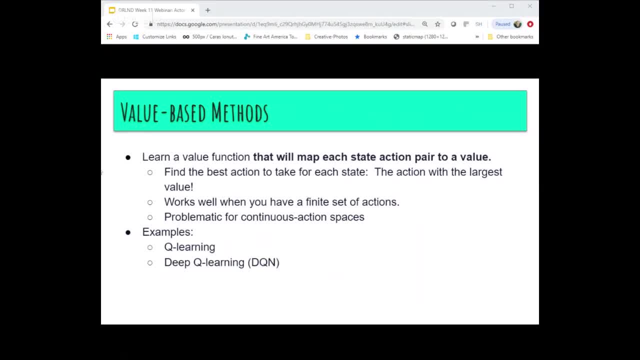 been talking about these different methods for a while. We started with value-based methods. If you recall, with the deep queue marketing and the deepvida manager, We studied what it was like to understand and formula of the internet economy through the basic information we have and then our routine, which is learning the secrets of 1957 with deep reinforcement learning. So now I'm going to come up with answers to some of the above points. that might include particular economic perspectives on leadership theory, More on this university learning objectives then, if it's easy to understand and fill in a bibliographic presentation. 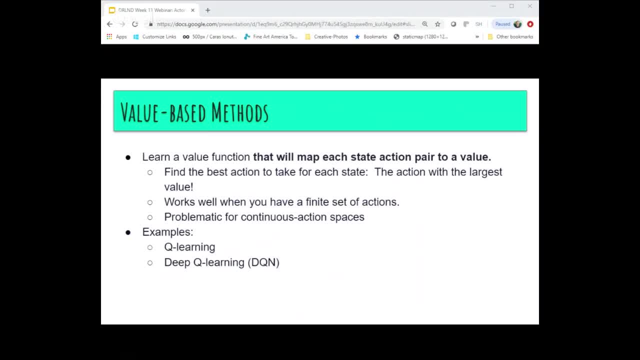 actually find some ways to understand what the work ofarnos x hat. nite 353 é elements to proceed with which deep queue network. if you have done the first project, you probably relied on this method to implement the first major project on the navigation project, and the idea in this method is that 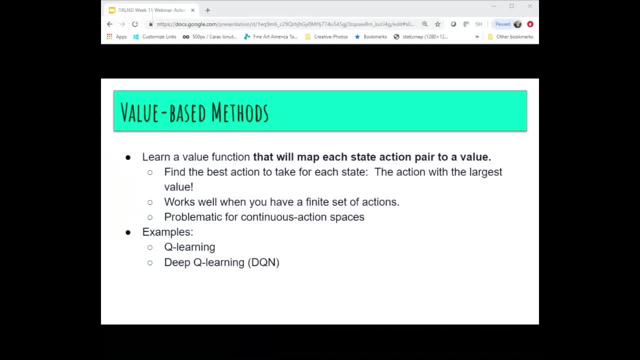 we train a neural network to learn a value function and then we use that value function to map each state value actually compared to a value and find in whatever state we're in we look at all the different actions that are available, the value functions that were estimated for each of those. 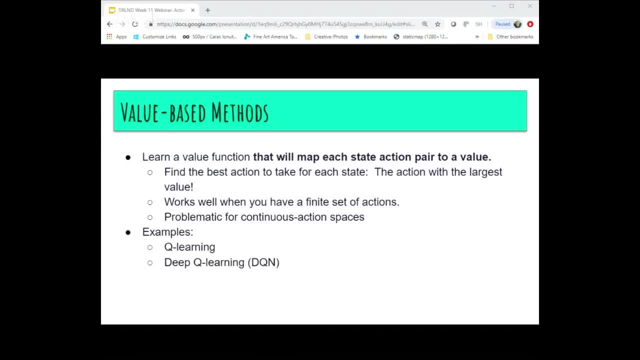 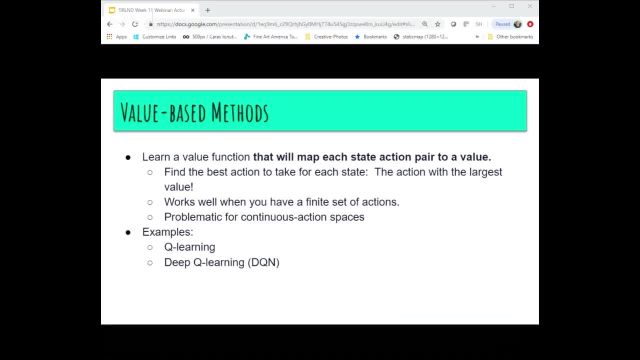 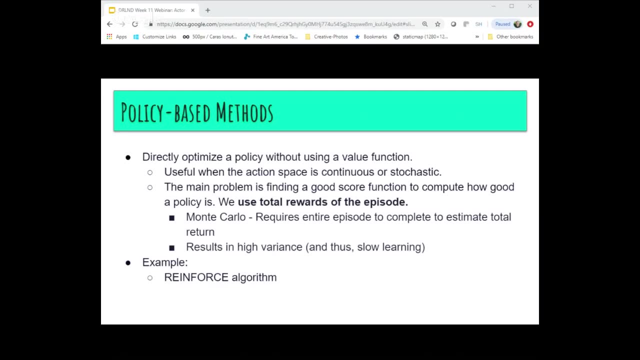 continuous action spaces. so, as i mentioned, deep q networks and q learning is a good examples of the value-based methods. then the next major type of algorithm we talked about recently are policy-based methods, and the difference in the policy-based methods from a value function approach is that 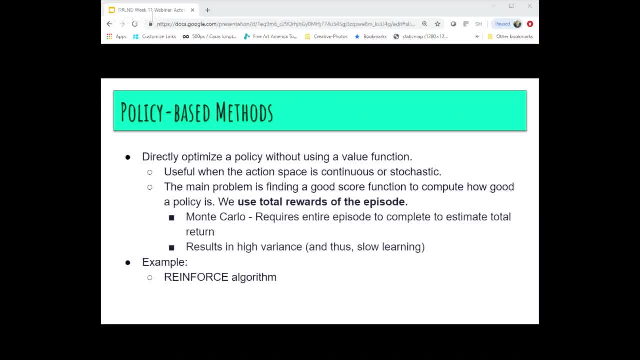 we directly estimate or optimize a policy without using a value function. so the, the neural network that's doing the, the function approximation actually is, is trying to find an optimal policy to select actions without first evaluating values of those actions. this, this approach we saw was, was good for a continuous action space or a stochastic action space. so there's a large class of algorithms. 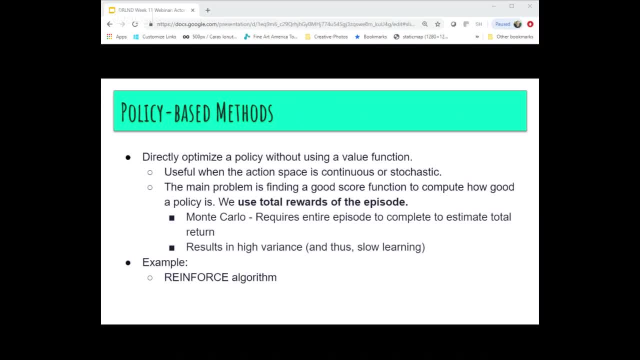 that require that type of approach. so policy-based methods can work well for that type of a problem domain. but uh, we thought we saw that, uh, a real problem with these types of methods is finding a good function. uh, to compute how good the policy is, and in in these initial techniques we use total rewards. 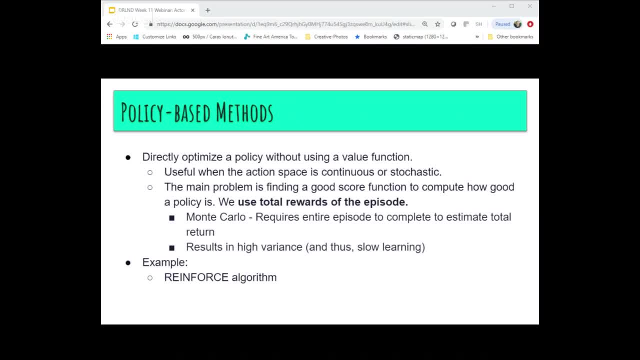 of the episode. it's a monte carlo technique, and the problem with that is that it requires you, to your agent, to actually traverse an entire episode, from beginning to end, before you can make any learning, before you have any learning take place. so so, because you do an entire episode, from episode to episode, actions that are taken. 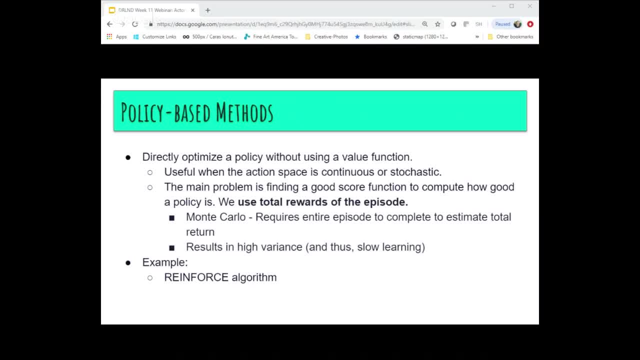 you know, at different points in the episode can have drastic changes in the final results and that results in high variance and that high variance produces what can oftentimes be slow learning. an example of this algorithm was reinforced that we talked about a few two or three weeks ago. 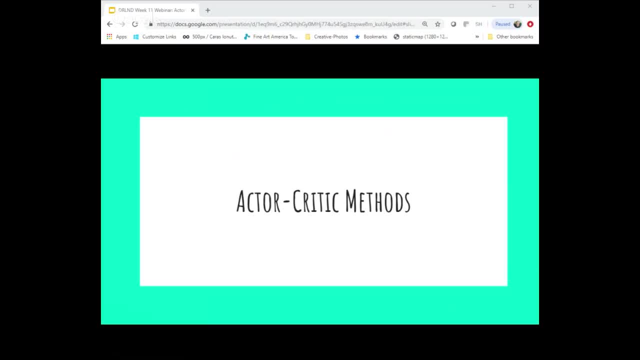 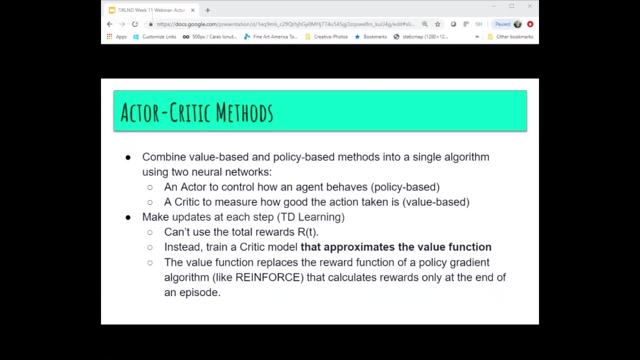 so, with that review of those two uh major classes of algorithms, let's talk now about actor critic methods. so the real uh idea is actually fairly simple. um, in actor critic methods, we combine both those methods we just talked about. we take a value-based method and a policy-based method. 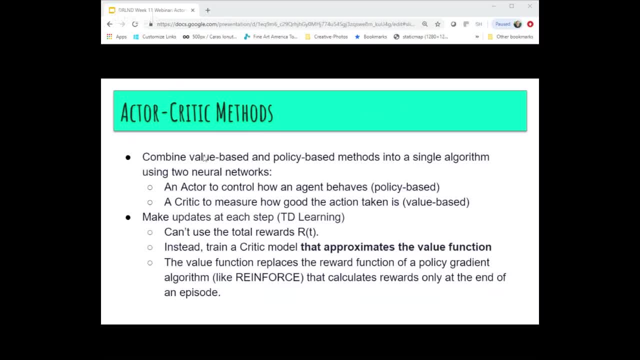 and put them into a single algorithm, use two separate neural networks. one neural network is an actor network that picks the actions. it controls how the agent behaves. this is a policy based approach. and then we implement a second neural network in the agent and this network is the critic. and the purpose of the critic is to measure how good the action that the actor 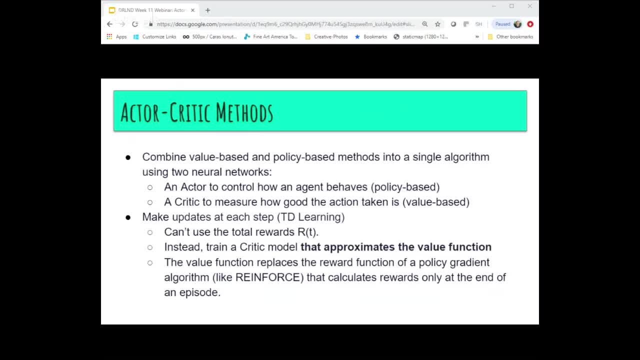 recommended to be taken, how good that action actually is, and this is a value-based approach. so we take these two, put them together in one algorithm and we overcome some of the, the uh, the problems that we solve with them individually, the the real main advantage of this approach is that 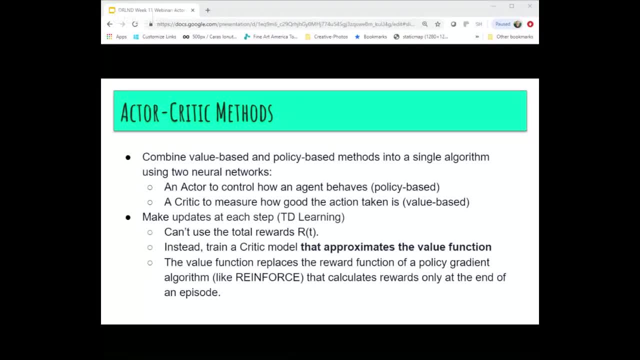 you can see that the learning is very different from the actual learning in the actual learning process and you can see, with this approach, that we've seen that we can do things in like the policy-based methods. we had these, a monte carlo uh technique, and we couldn't do learning until. 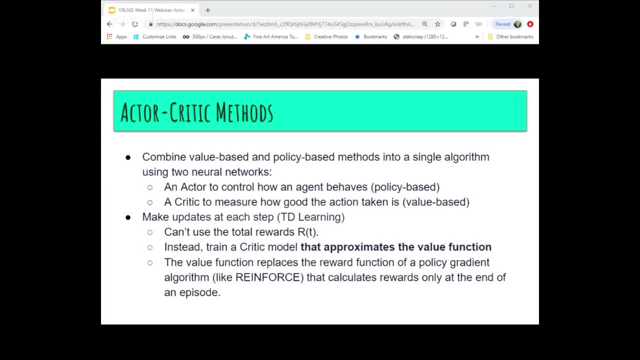 we completed an entire episode with an actor critic approach. we can make updates at each time step. we can make learning activities take place every time we take a step in the environment. this is a temporal difference learning approach and we've seen how that can be advantageous because it reduces variance in learning. 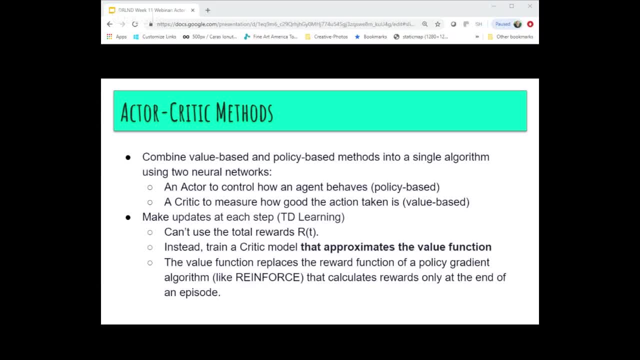 the critic model to approximate the value function. Value function replaces the reward function that we saw in, like the reinforcement algorithms policy gradient, that in that method only calculated words at the end of the episode. But here we can calculate those rewards and take those rewards into account and take a learning step with every step we take in the 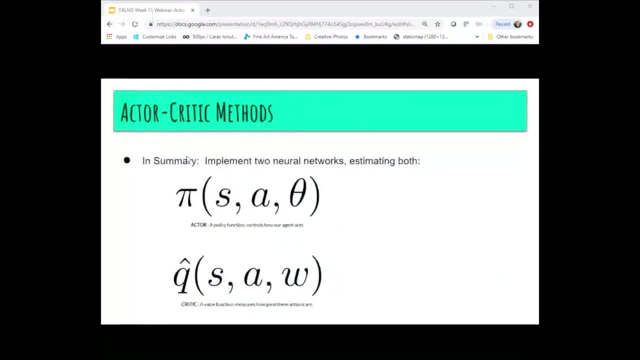 environment. So really that's the kernel of the entire method. So, in summary, we implement two different neural networks In reality. I should mention that often you'll have more than two neural networks because you'll see in the standard algorithms, starting with the deep deterministic, 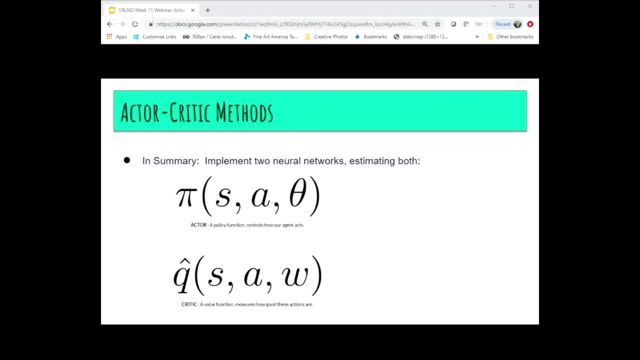 policy gradient algorithm that you'll use in the last two projects, that each one of these main neural networks has a sister network that goes along with it. It's a soft update where you can see what's happening in the environment and what's happening in the environment. 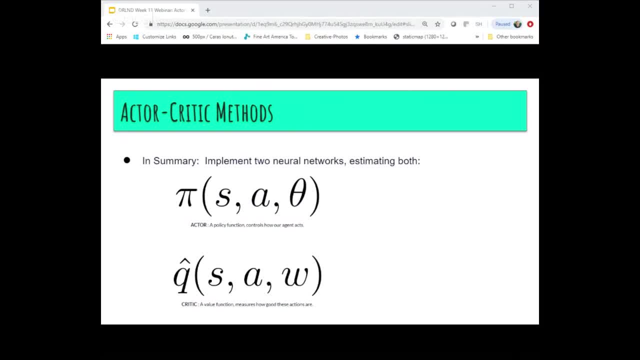 Process, and that soft update process lets you take actions on a policy that doesn't change very often And then slowly update that policy based on the learning that takes place in the more rapidly changing primary neural network. So in any case, there's two main neural networks: the policy- 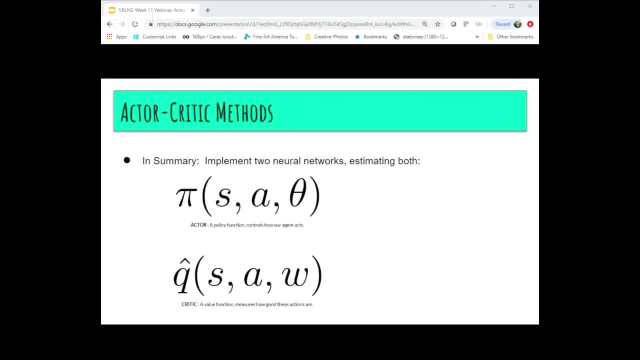 network that's implemented as the actor and that controls how the agent acts. it selects the actions And you can see it's a function of the state that you're in, the action that you take and a set of data values that are the weights of the neural. 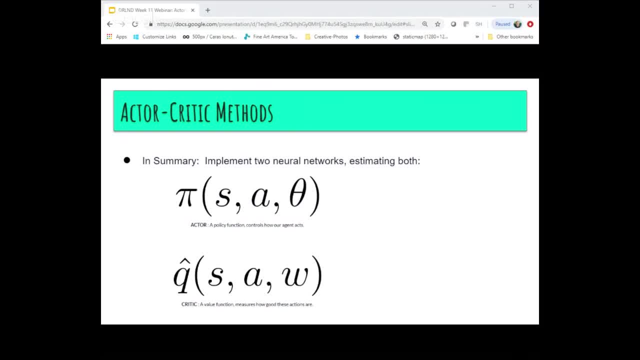 network, It's the policy network. Then there's also the second network, it's the critic network, And this is a value function approximator and it measures how good those actions were that were recommended by the policy network And this Q function, critic network. 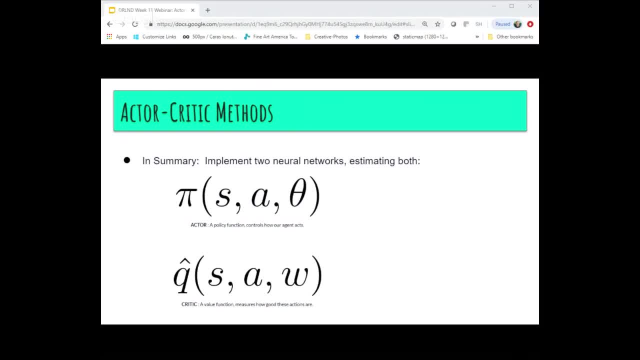 sometimes it's a Q function, sometimes it's an advantage function. Q hat kind of is a generic value function here, But in this case it's based on a state and an action and a set of weights, And the weights- W or omega- here are the weights of that critic network. 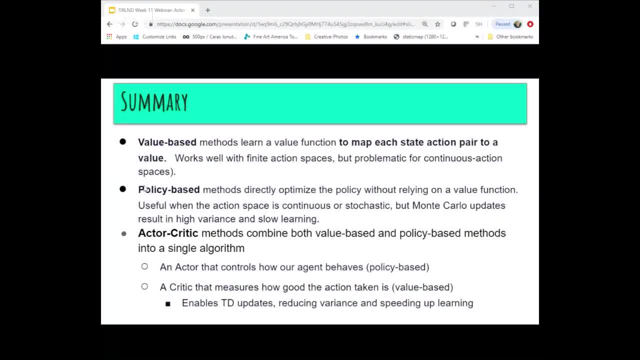 So, in summary, today we talked about two of the earlier methods that we've discussed in the course- value-based methods that map each state action pair to a value, And we talked about how those work well with finite action spaces. But we talked about how a number of these methods are problematic for environments with continuous 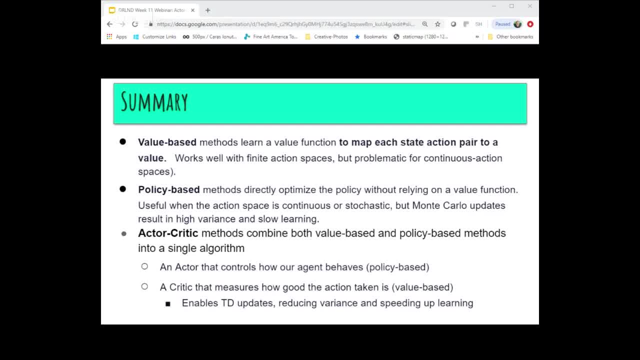 action spaces. And then we reviewed the policy-based networks that directly optimize a policy without relying on a value function, And those methods can be used in continuous or stochastic action spaces. But the problem that they had was that the Monte Carlo learning updates require you to complete an episode before you have a step of learning, and that resulted in high 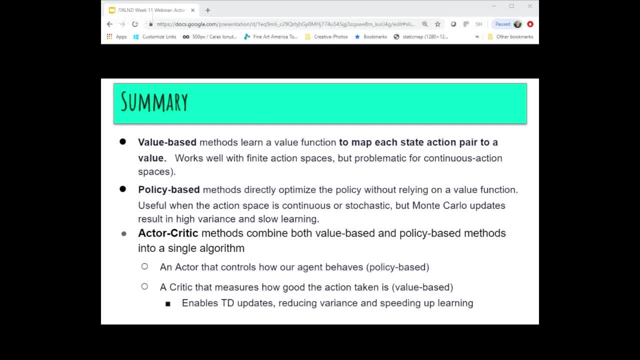 variance and slow learning. So in the actor-critic methods we combined the two methods and we found the results in the context, those two standalone methods, the value-based and policy-based methods, and put them into a single algorithm. the actor part of the algorithm controls how the agent behaves. that's the policy-based. 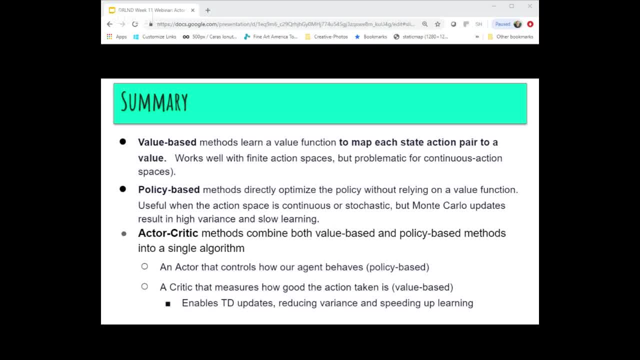 part of it. it picks an action based on the state that you're in, and then there's a critic that measures how good that action is- and it's a value-based method- and the actor critic. the version of the critic that's used in these algorithms enables temporal difference updates. 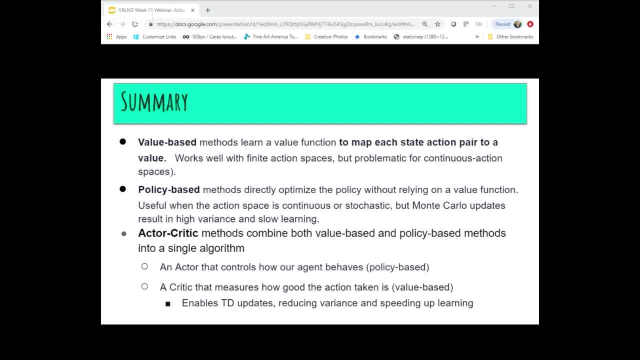 and- and that gets by the, the high variance we saw in monte carlo- update methods with standard policy-based approaches and with that we can reduce variance and speed up learning. so you know- i mentioned the beginning of the talk- that these methods are important: the- the actor critic methods.